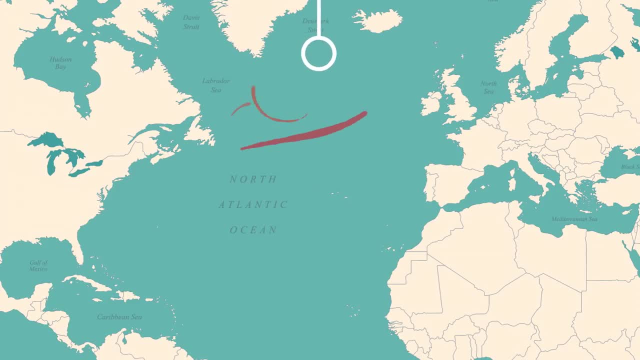 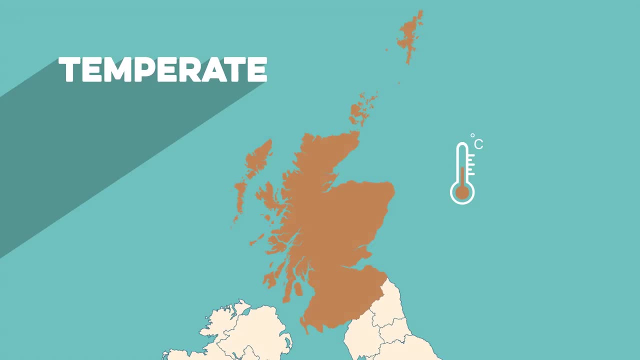 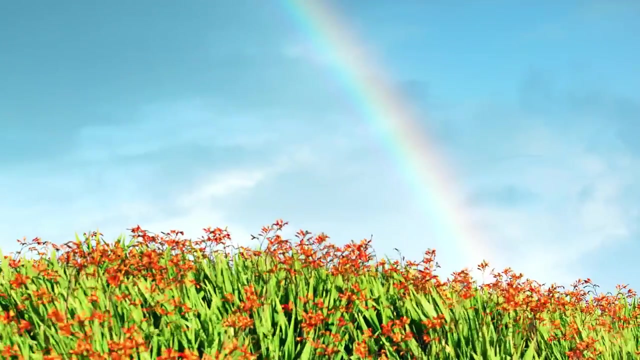 swells produced by the Gulf Stream. In simple terms, the effects balance one another out, which leaves Scotland with what is known as a temperate maritime climate. What does that mean exactly? Well, it means that, while Scotland's weather is unpredictable, 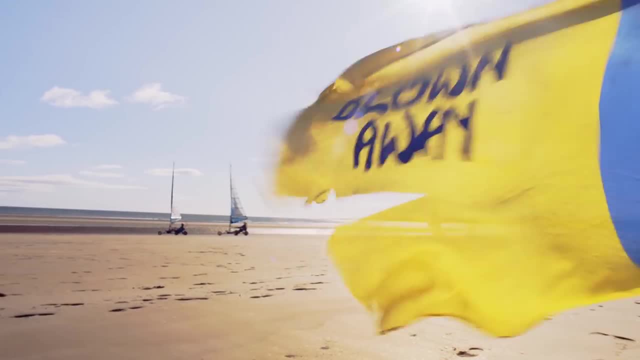 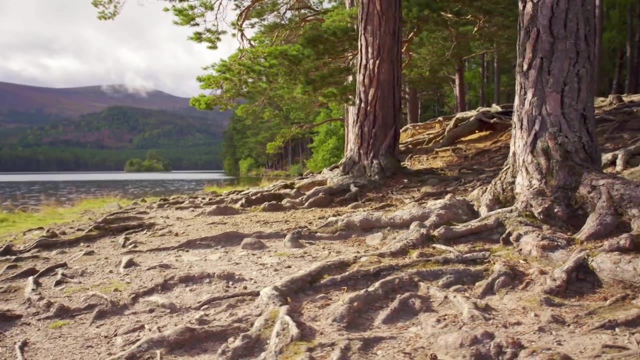 it is very rarely extreme. Thankfully, we don't need to worry about hurricane season here. Think cooler than bitterly cold, mild rather than baking hot. So wherever you're headed, bring a coat and remember what a wise Scotsman once said: if you don't like, 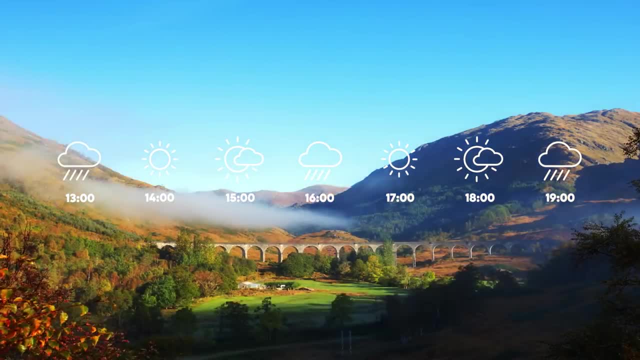 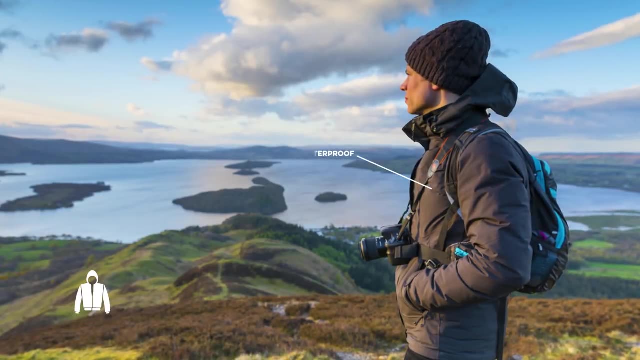 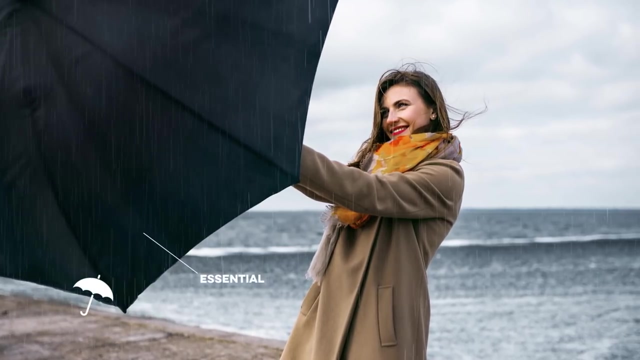 the weather. just wait five minutes, Be prepared. Here are some key items: A fully waterproof raincoat complete with hood to shield you from rain and drizzle. An umbrella is an essential piece of kit, Perfect for mild days when you don't want. 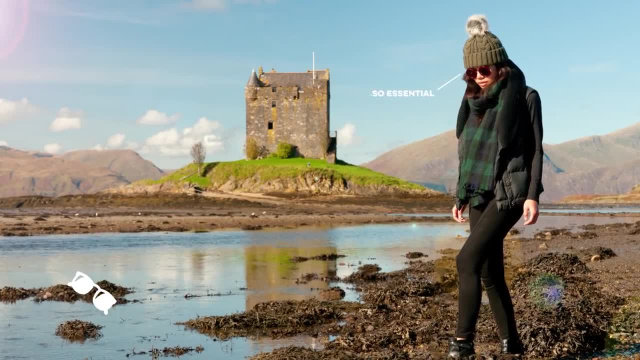 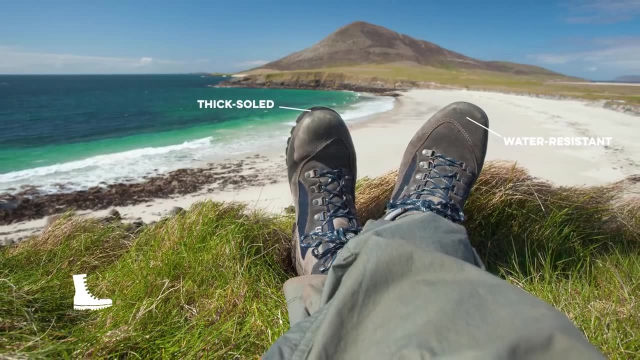 to be caught off guard. Don't forget your sunglasses. You may well use them as much as your umbrella. A durable pair of thick-soled, water-resistant boots. Athletic shoes are great for the summer, but a pair of stout hiking boots are essential for exploring the 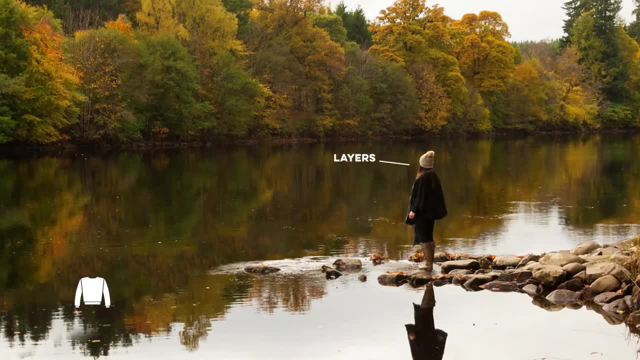 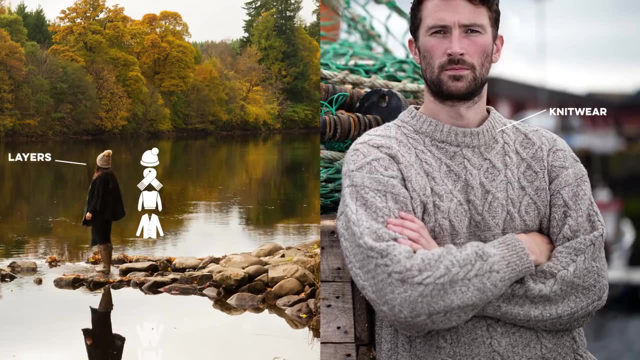 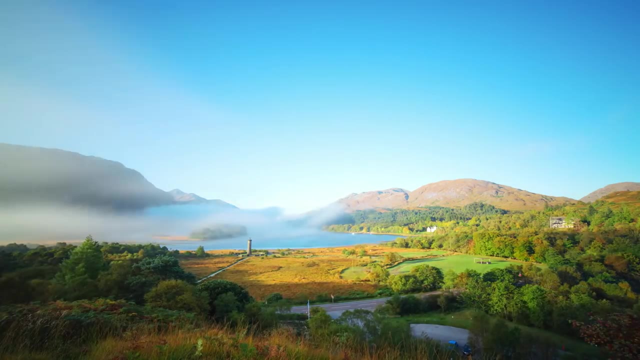 great outdoors. The key to dressing in Scotland is layers. Bring plenty of t-shirts and a snug jumper. Naturally we recommend Scottish knitwear, but then that's just our humble opinion. There are many perks to our changeable weather and unique climate, like atmosphere, Blue. 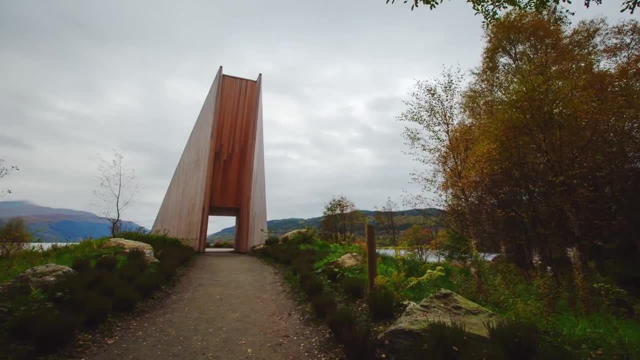 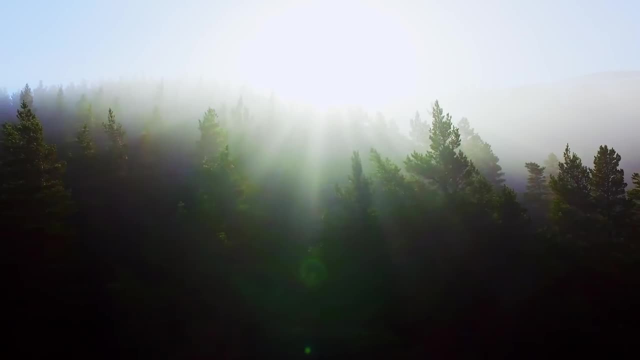 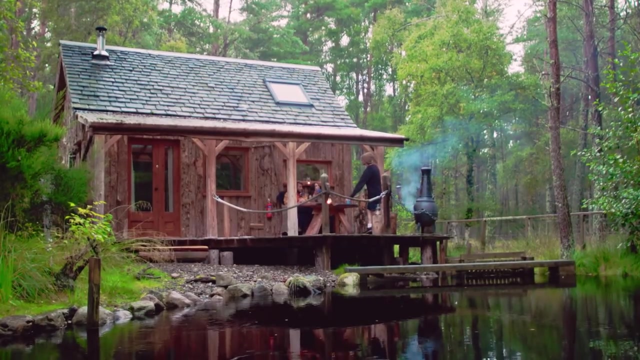 skies are lovely, but when it comes to mysterious, dramatic backdrops, we believe that the weather is all part of the drama. Contrasting clouds and ethereal mist are all part of the magical spectacle people flock in their droves to witness. Scotland is endless proof that even the rainiest day can be beautiful. 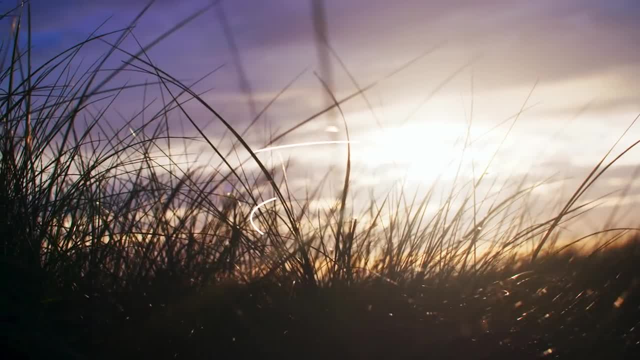 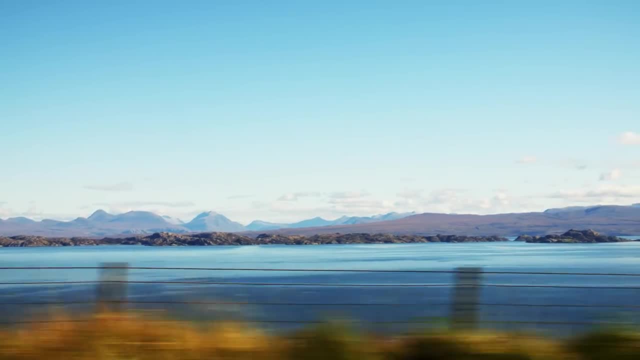 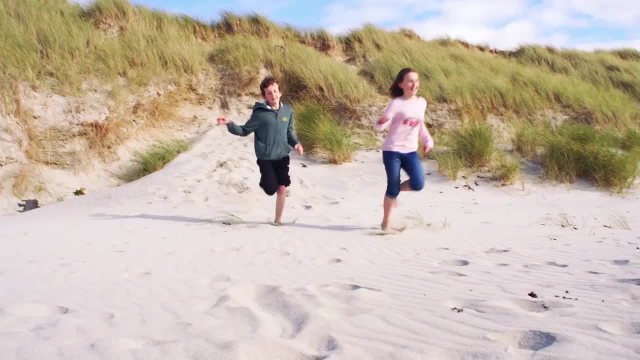 The weather is always a good sign of a good day. The weather is always a good sign of a good day. You can get to the beach from the layworks. further north you go, Making this a prime time to visit the northern Highlands and Islands.